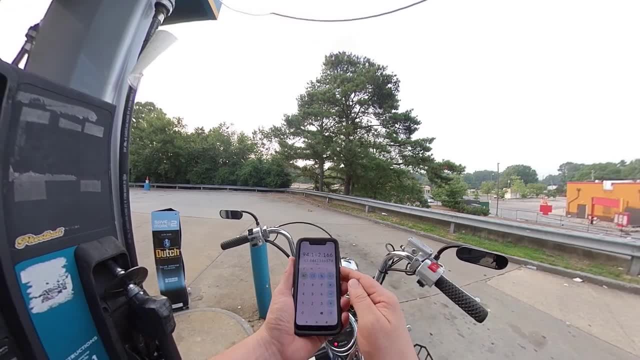 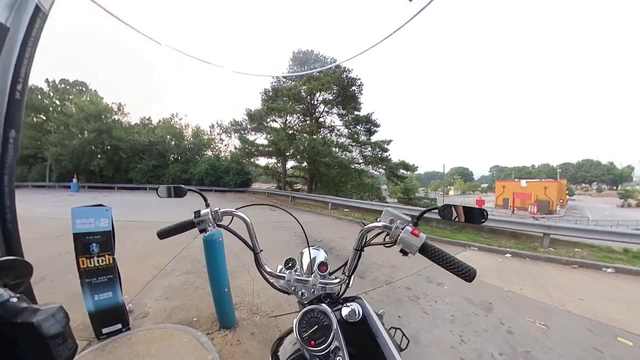 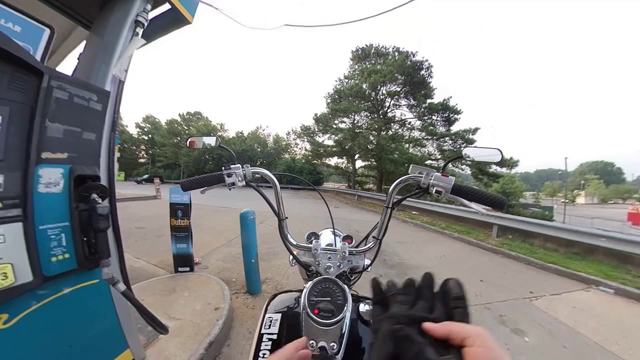 gallon. all right, remember this number. we're gonna need it for later. and then, once you're filled up- i forgot to mention it before. sorry, but go ahead and clear your tripometer, reset that guy to zero and go ride some more. you're gonna want to do this probably two or three times, because you're gonna want an average. 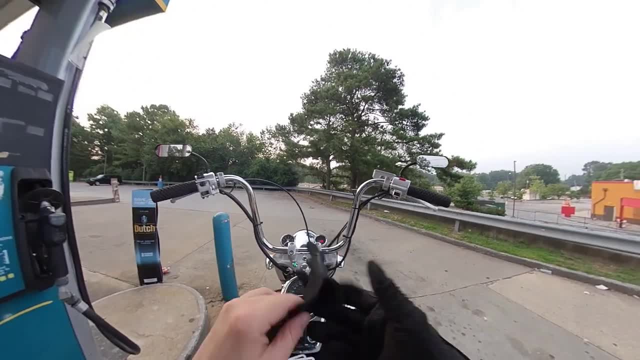 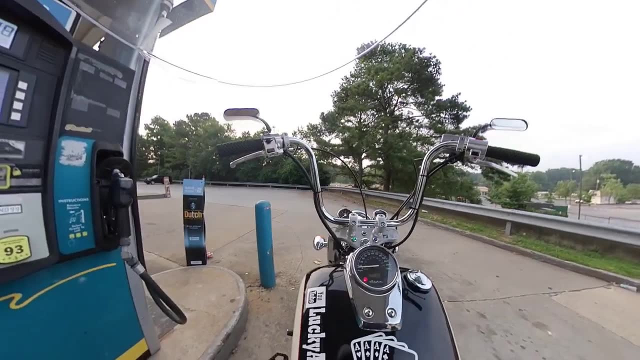 and i highly suggest driving just how you normally would. so if you spend an hour on the highway every day, just do i mean, do you know, do your normal routine? all right? so now let's look up the fuel capacity of our motorcycle. so for me, i'm gonna type 2008. 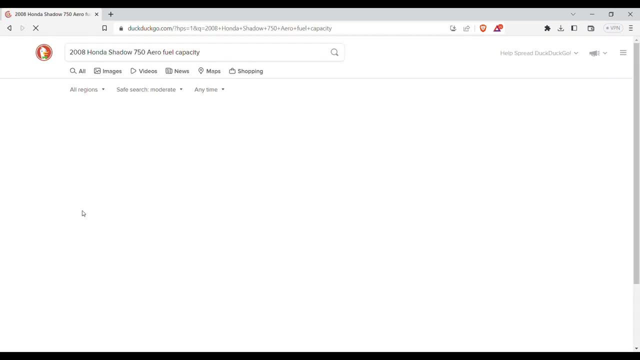 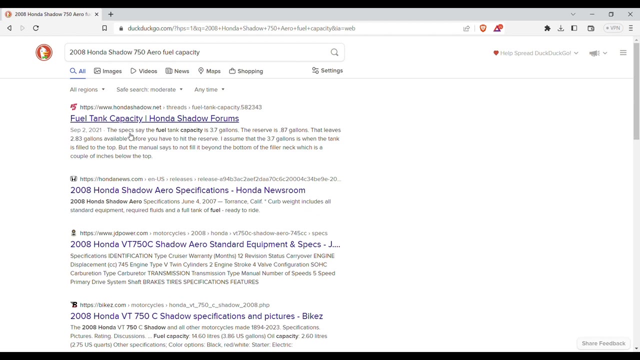 honda shadow 750 aero fuel capacity and see what that comes up with. so the first result here is actually from one of the internet forums and you can see someone references 3.7 gallons. but i'd much rather go with a more reputable site. usually i use bikescom. 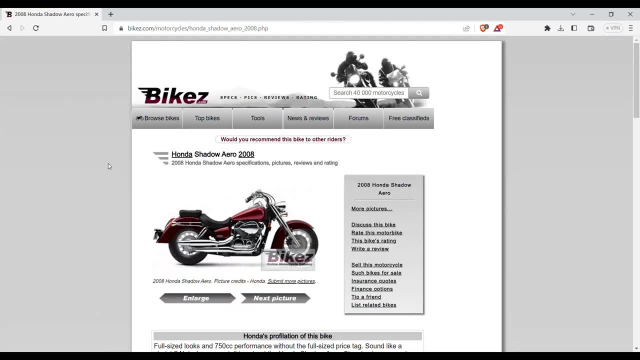 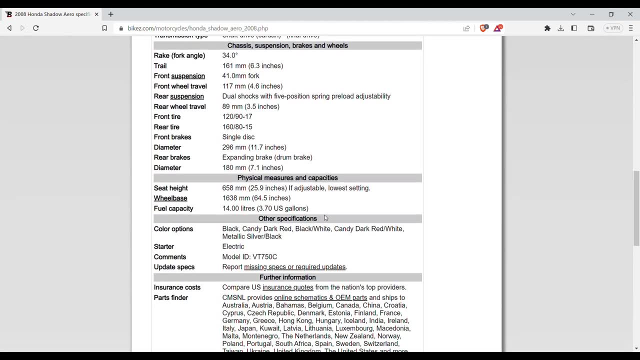 as they seem to provide a whole lot of information. as you can see right there, honda shadow 750, arrow 750. scroll down a little bit. it gives you all kinds of information, but that's what we're looking for right there. so now we know the fuel capacity of my bike is 3.7 gallons. 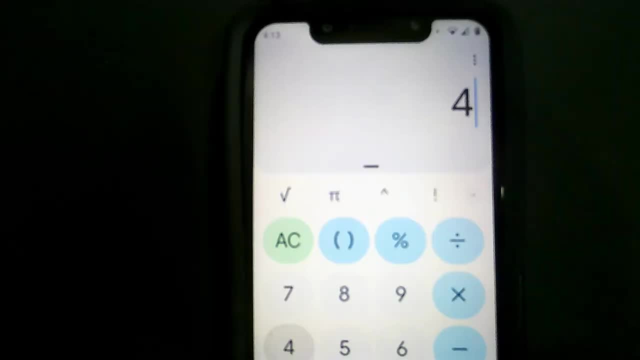 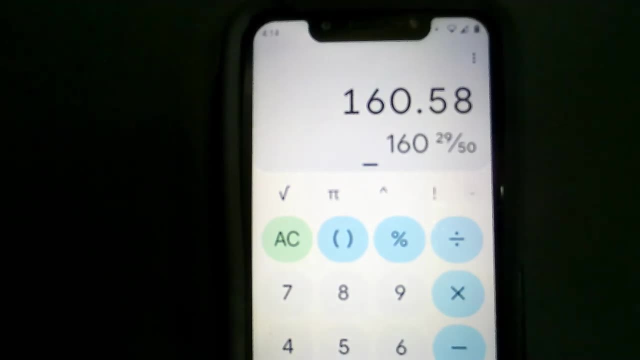 take our 43.4 from earlier. i'm going to multiply that by our 3.7 and there you go. so i know, on my 2008 honda shadow arrow 750, it has a total range- and i mean like every drop in that tank- of 160.58 miles. so probably when i 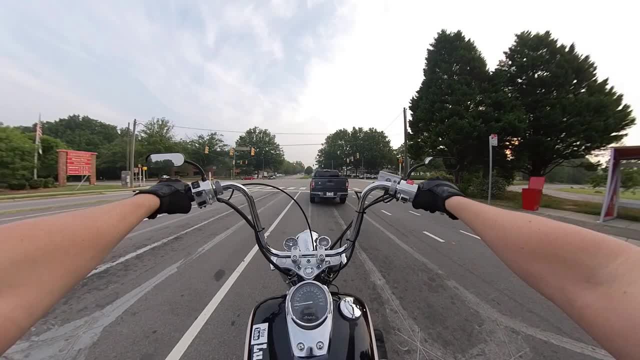 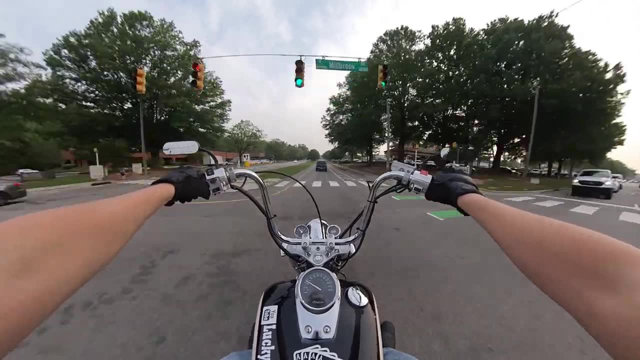 hit 120, i need to know. i need to start looking for some gas. so if you don't have a fuel gauge, you can always use your tripometer. it's actually a lot simpler than you think, so hopefully this video helps some of you out. i wanted to put this out there. i mean, it seems like such a simple thing. 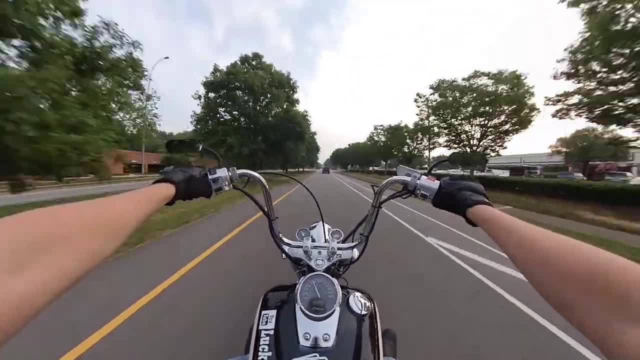 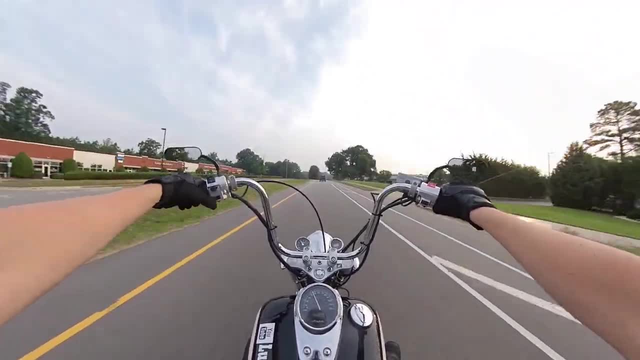 but i do see it getting asked- uh, quite a bit online, so i just thought we should talk about it. mainly, i just didn't want you guys to be a dummy dum-dum like me and run out of gas like i didn't. you know this video here, so until next time, y'all be good. see ya.